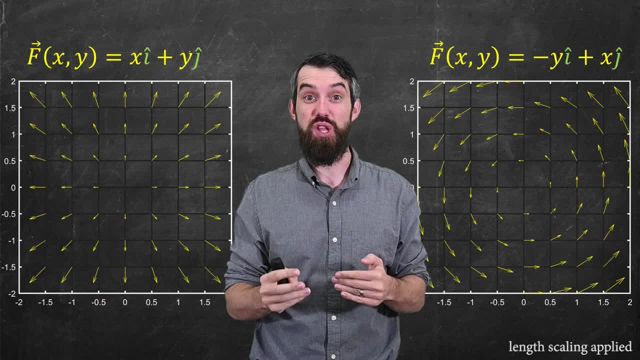 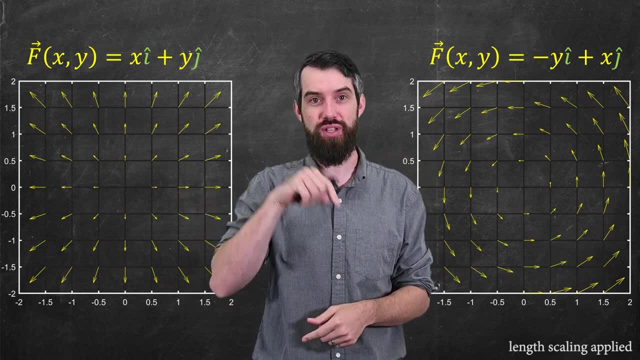 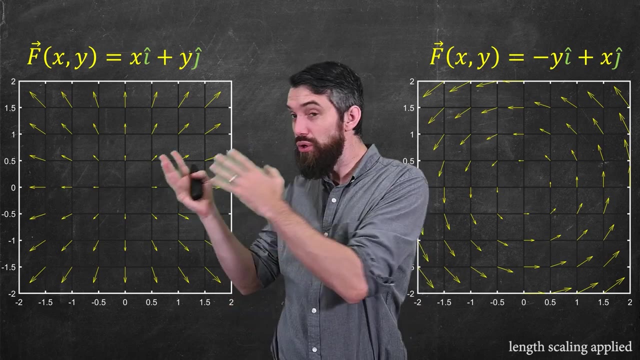 In this video we're going to talk about flow intervals and circulation. This video is part of my larger playlist on vector calculus. The links to that playlist and all my other courses are down in the description. Now, what I want to begin with is contrasting two. 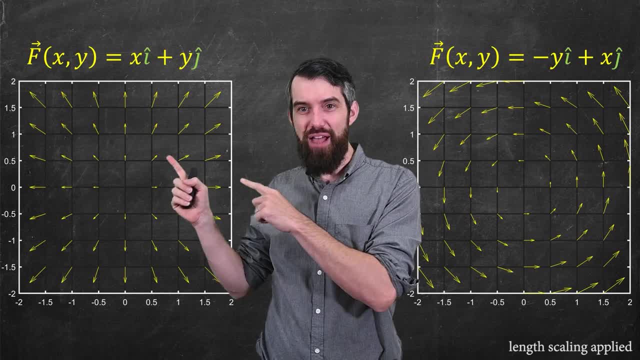 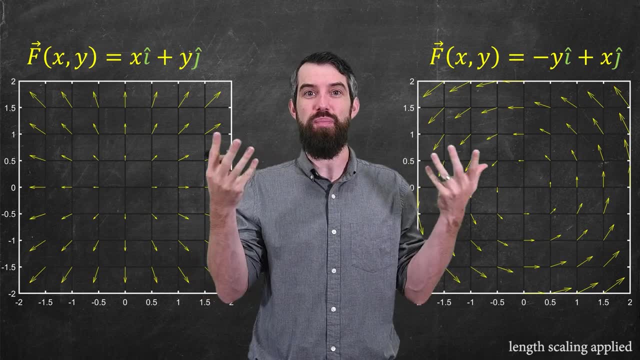 different vector fields. The one on the left, who's given by the equation x i hat plus y j hat, has the property that everything is dispersing from the origin, That is, at any point the direction of the vector field is directly away from the origin, Whereas the 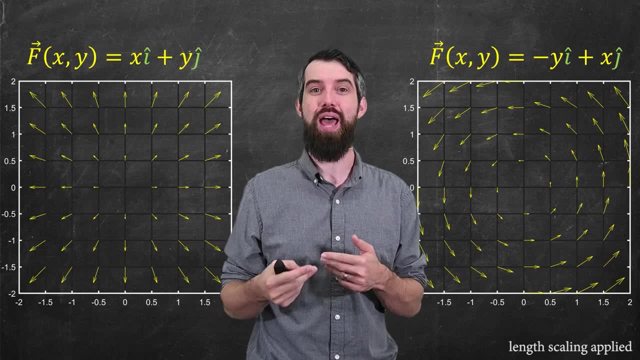 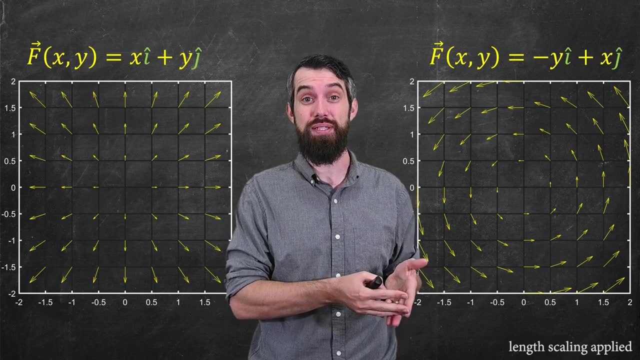 one on the right here which is given by minus y, i hat plus x, j hat is a spin field. It has this behavior where everything appears to be rotating counterclockwise. Now so far in vector calculus we've seen that vector fields can have a bunch of different physical 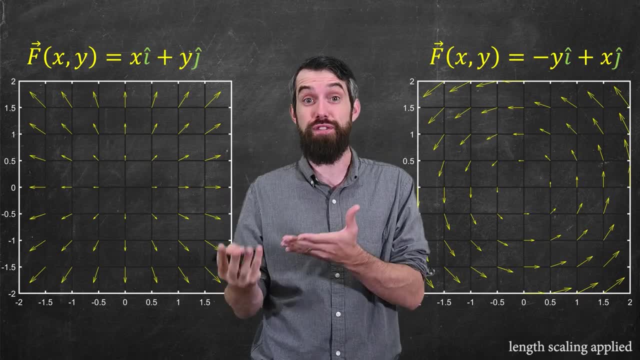 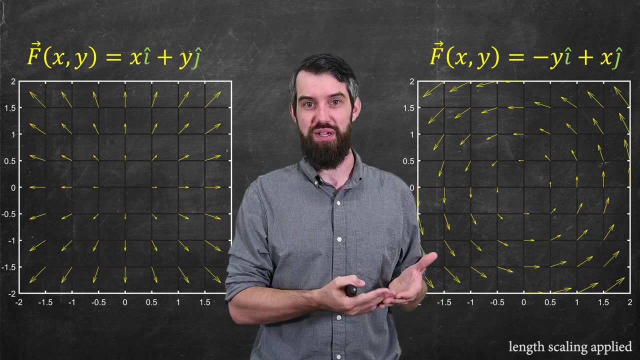 interpretations. For example, we've seen that it could represent a force field, like the force field that comes from gravity, But in this video we're going to imagine these vector fields represent velocity fields, For example, in some turbulent water system or turbulent 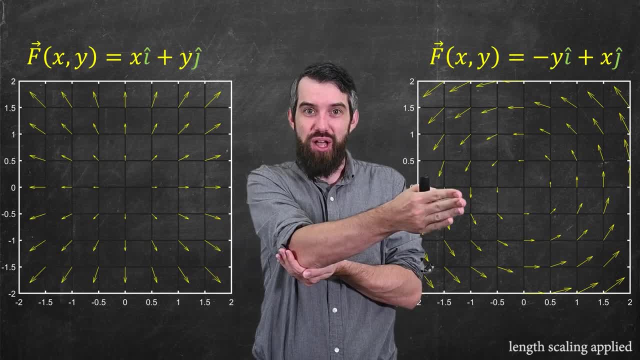 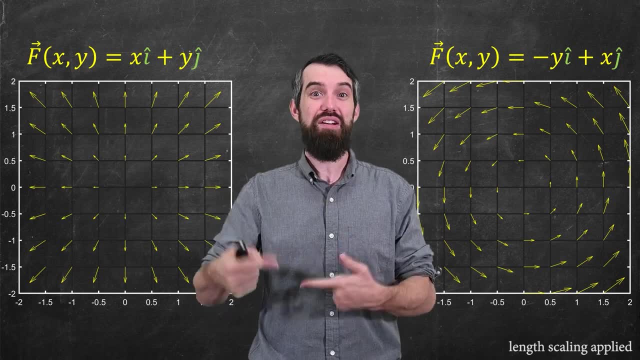 wind system. you have a point and then the vector tells you the magnitude and the direction that either the wind or the water is flowing at that particular spot. And thinking of these vector fields as velocity fields is going to really build some physical intuition, for 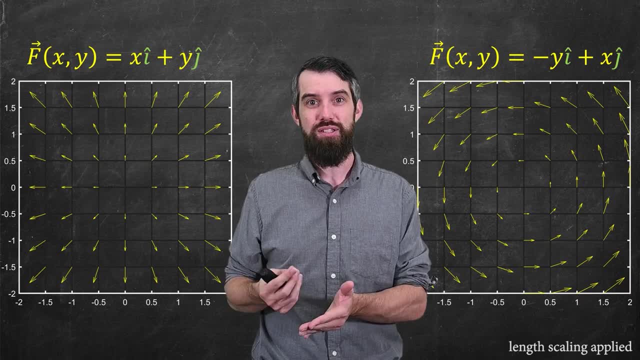 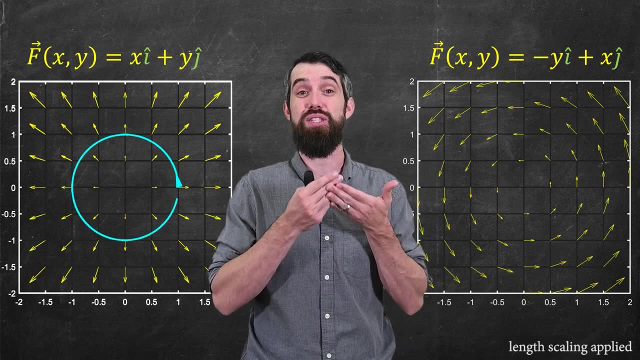 the concept we're going to introduce in this video of flow and circulation. So now I want to show you something very different. Let's imagine you take some path that goes through this vector field. It goes around in a counterclockwise circle, And I'm going to do the same thing. 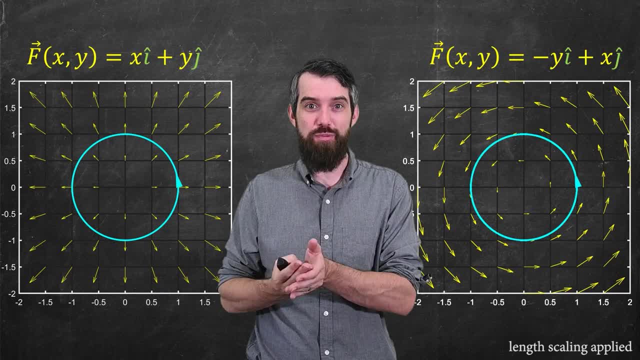 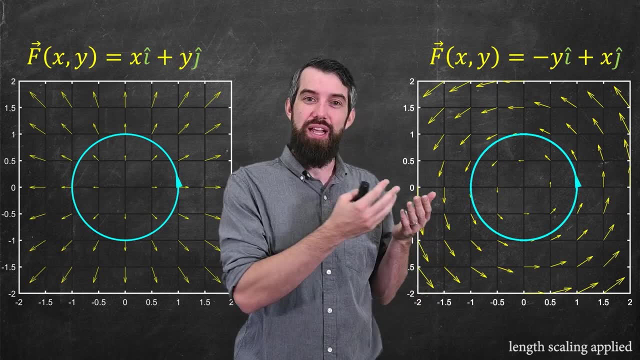 for the other one. In other words, I have this same basic path but in two different fields. Now there is a difference between these two cases. For the spin field, the path sort of aligns with the vectors. You can imagine, for example, if you had a spinning. 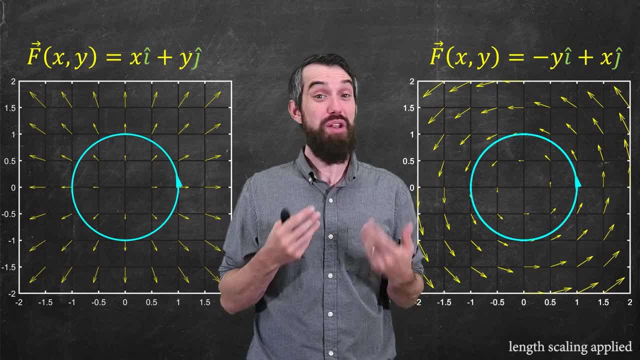 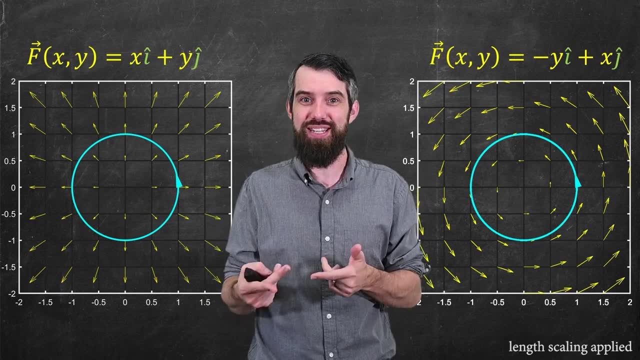 body of water and you were just paddling your canoe in it. Then you could imagine if you wouldn't have to paddle your canoe at all because the velocities of the water was going around in a circle and the path you wanted to take was going around in a circle. You would 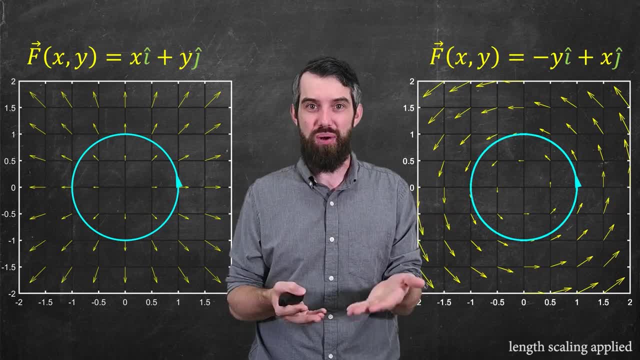 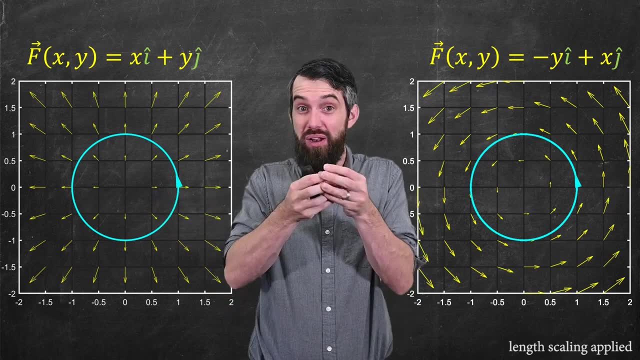 just thus not do anything and the water would move you around in your circle, Whereas if you're in this field, that's sort of more of like a source, like I could imagine, for example, a water fountain in the middle and then everything disperses away. Well, it would take a lot of work You have to do. 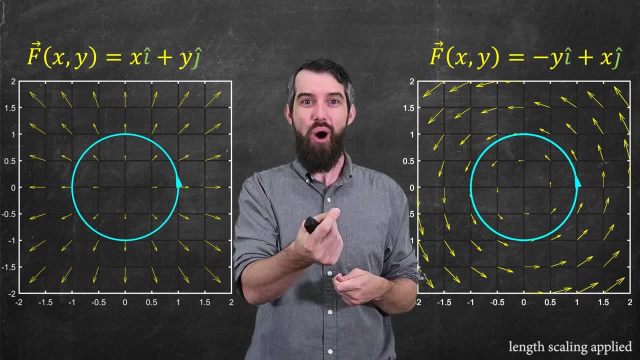 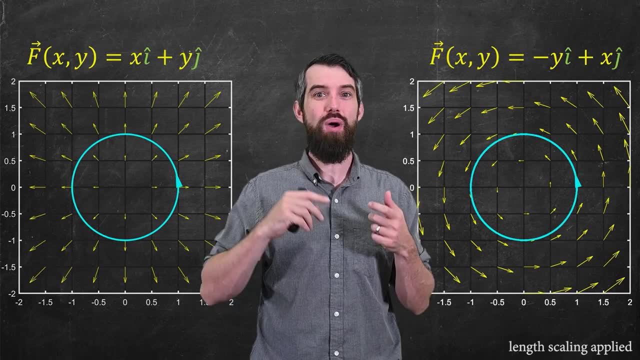 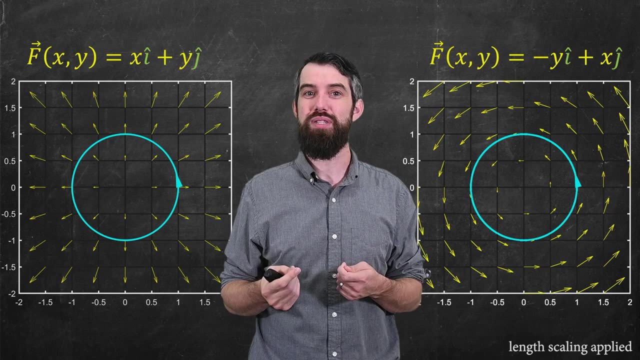 a lot of paddling to actually be able to travel in a circle, because you'd always be going orthogonal to the velocity field of the water that you were paddling in. So I want to capture this concept, I want to figure out some notion that I'm going to call flow, and flow is going to represent the 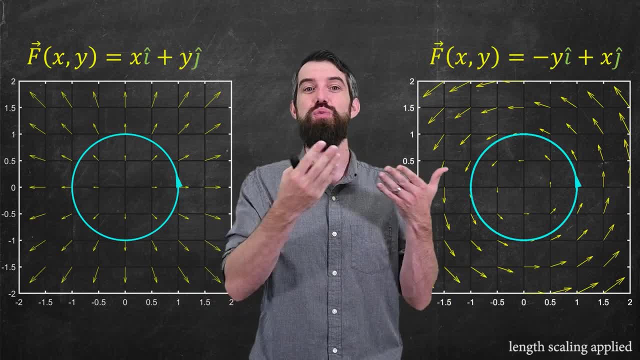 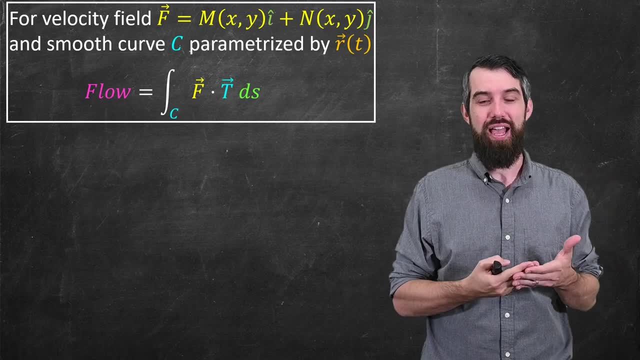 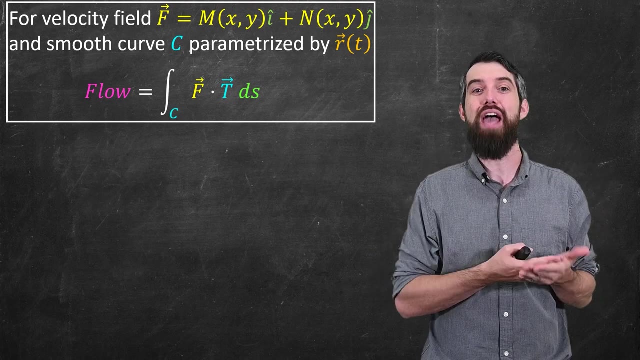 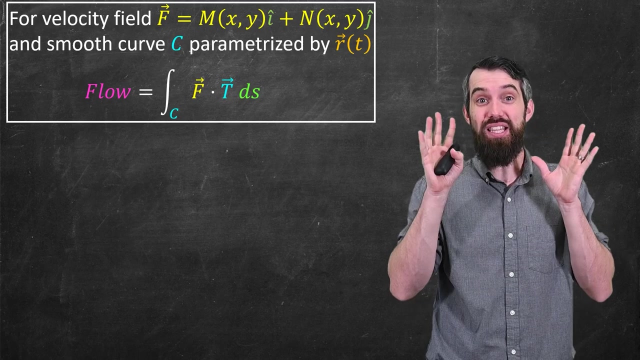 degree to which my path is aligned with the vector field. Okay, so here's our formal definition. It says: if you have a velocity field f and a smooth curve c, then the flow interval is just the line interval Of f, dot, t, ds. Now what you might observe is that the formula I've given here is exactly the 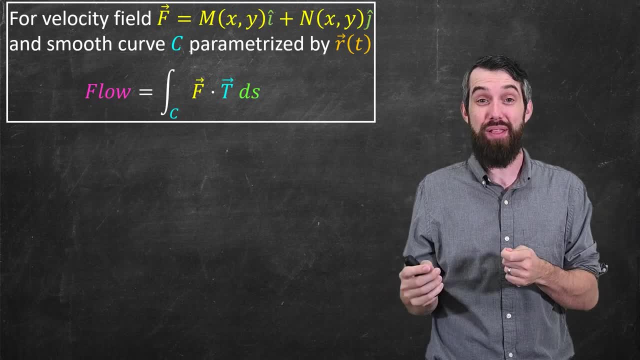 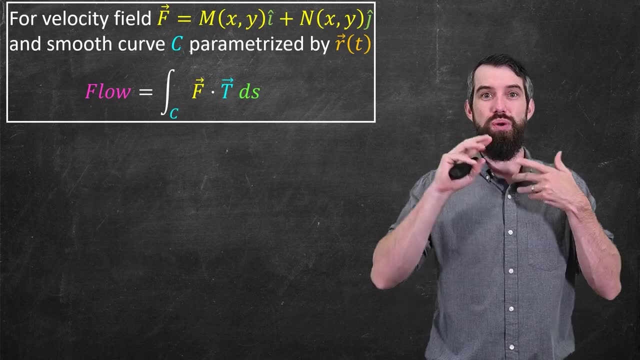 same formula. There's nothing new about it- as the formula that I gave when we talked about work done by a field on some particle moving along a path. So the actual line interval, the mathematics of it, is the same. What's changed here is the physical interpretation. Again, if I look at the 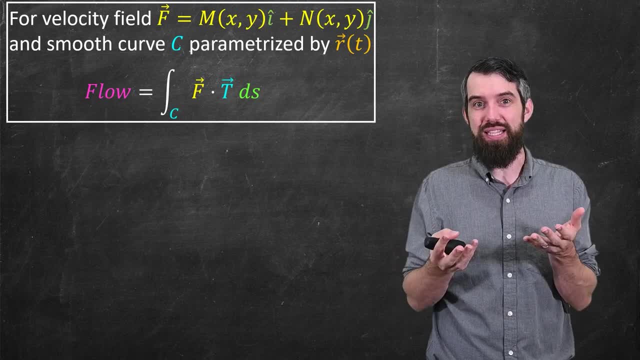 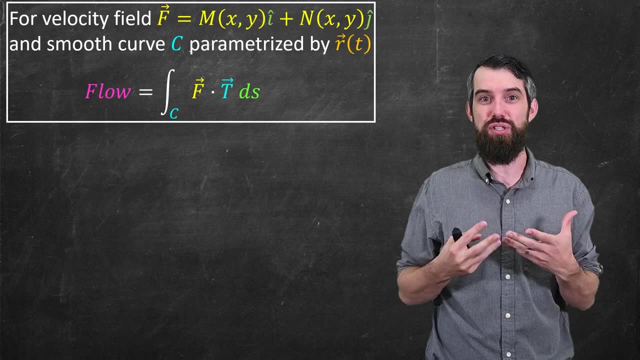 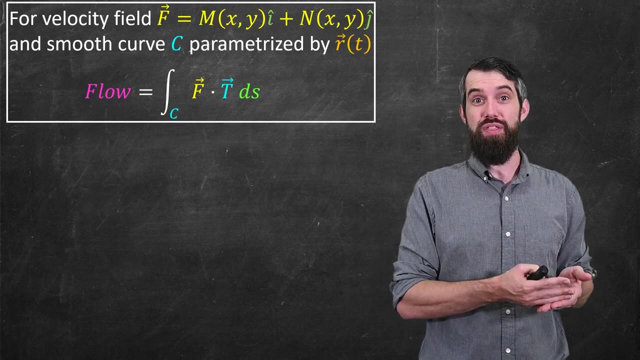 integrand what I have when I look at the f dot t is I'm saying, well, f dot t is the tangential vector to the curve. I'm saying I want to add up the contributions of the field in that tangential direction. Now, as we've seen before when we looked at, say, work, this: 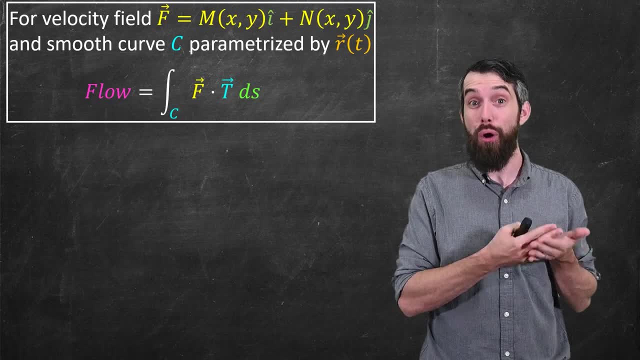 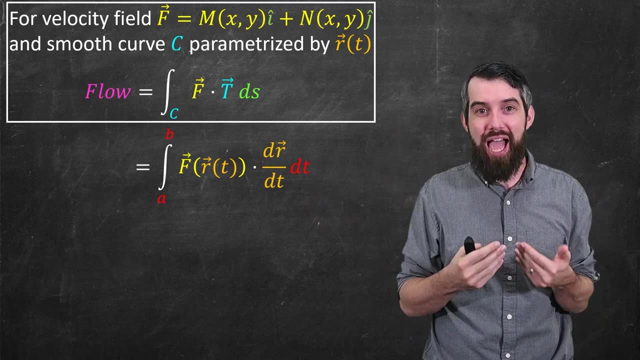 formula is a great definition, But if we're given an explicit r of t, a parameterization for the path, we need a way to compute it. So, exactly as we've seen before, we get the parameterized version of this formula. So it's the interval from a up to b If your path is parameterized where t is going. 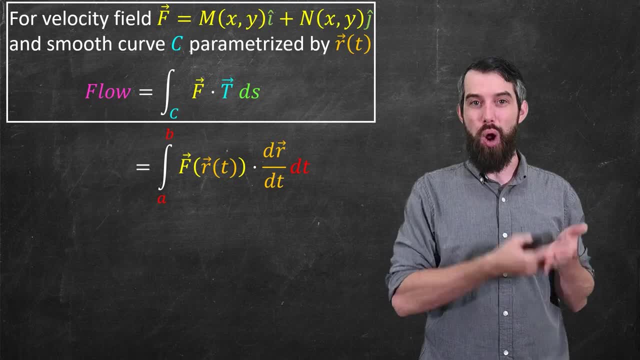 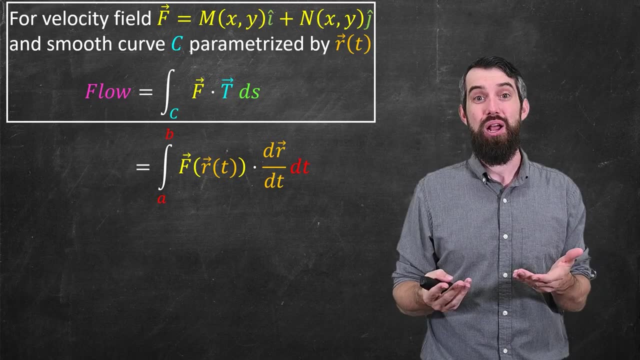 between a and b Of f dot t, ds Of f of r of t dotted with r, prime dt, And so thus, if you know your field and you know your r, you can just plug it into this formula to compute it. We've also seen in the video online integrals: 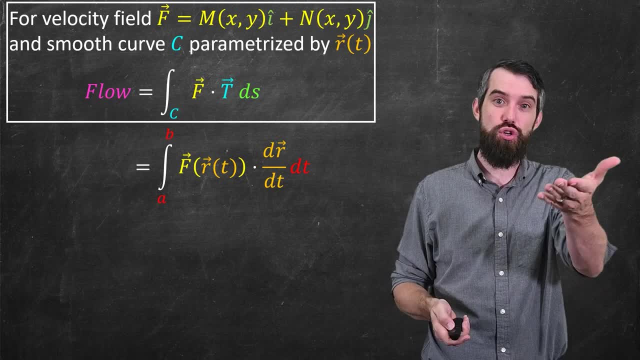 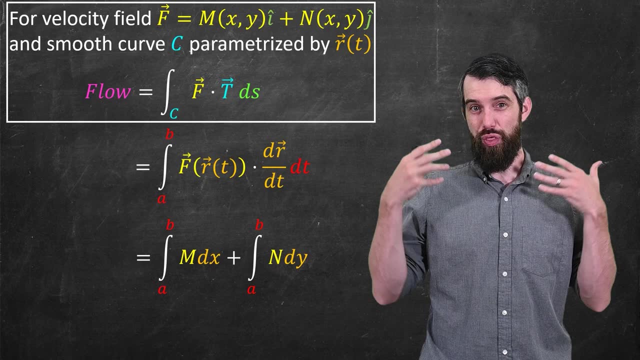 with respect to x is that we can rewrite this in a new shorthand. We can just call it the integral of mdx plus the integral of ndy. I often like remembering this third version of it. It's sort of a shorthand. I think it's really simple. I just plug in the m and the n And then I have to. 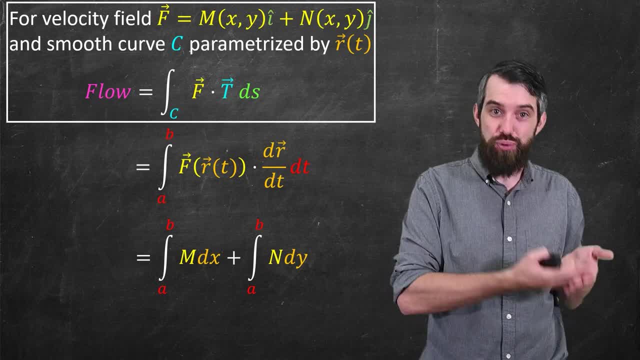 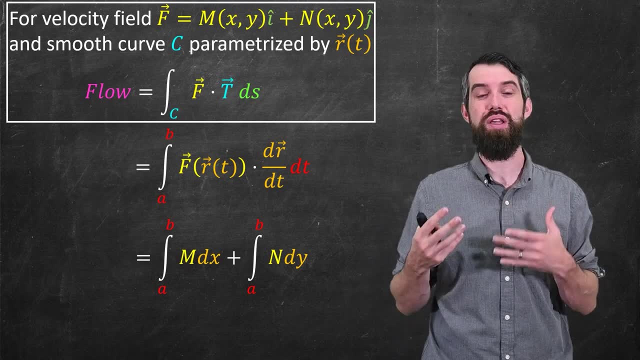 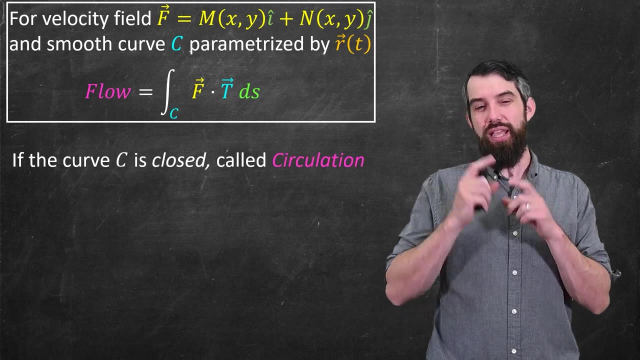 remember, the dx and the dy dy are always going to be g prime of t dt and h prime of t dt respectively. So regardless whether you use the second or the third equation here, these are what you use to actually compute it. Final bit of terminology is: this is just a general curve, But if the curve is closed, 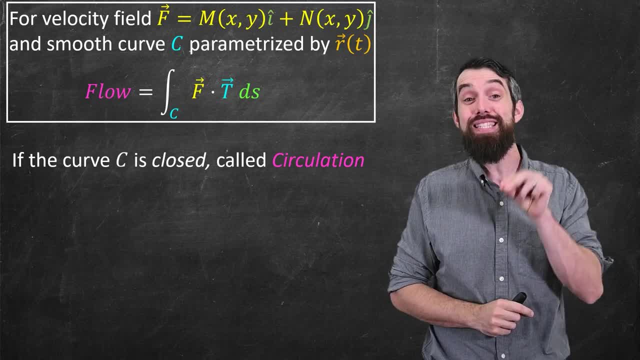 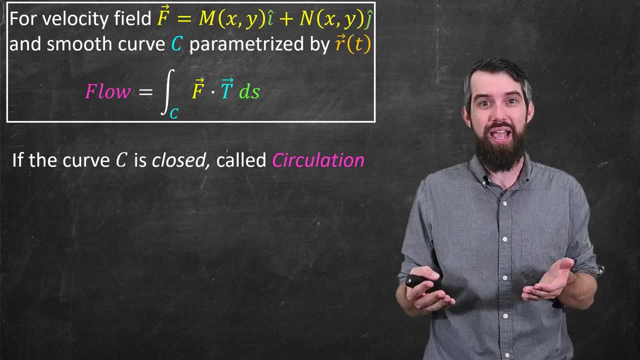 and what I mean by closed is a curve that ends up exactly where it started. So, for example, the standard curve is just the circle going around with t between zero and two pi, And then the curve is closed because the value at t equal to two pi, the end is the same as the. 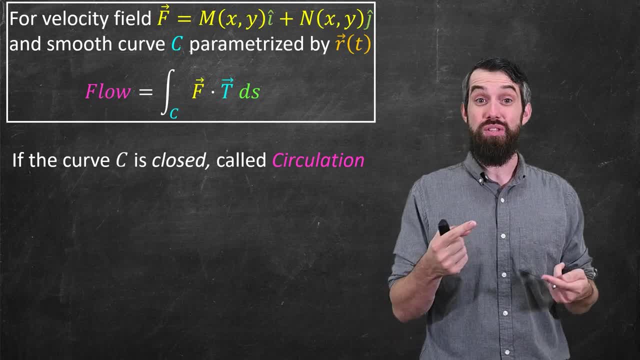 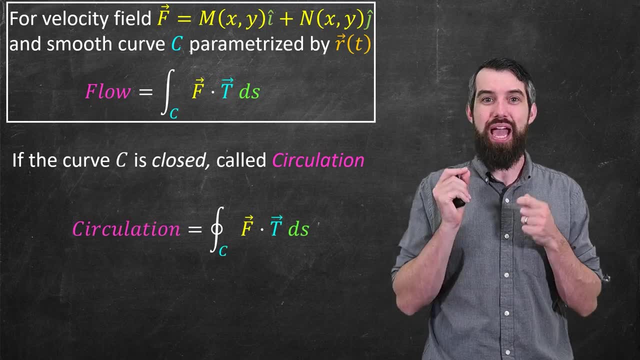 value of t equal to zero. the beginning. Anyways, when your curve is closed, we give it just a new word. The flow interval is called the circulation, And to indicate that we add a new symbol. So it's the exact same formula, except our integral sign has this little circle inside of it And that 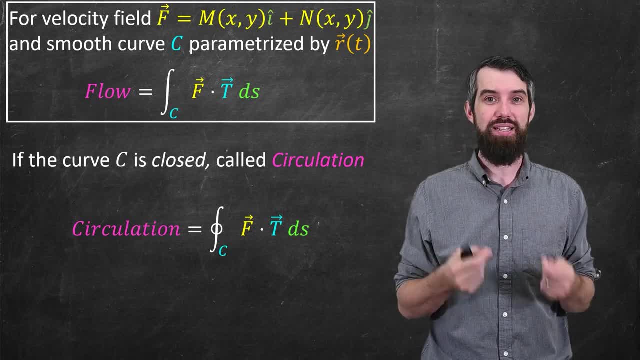 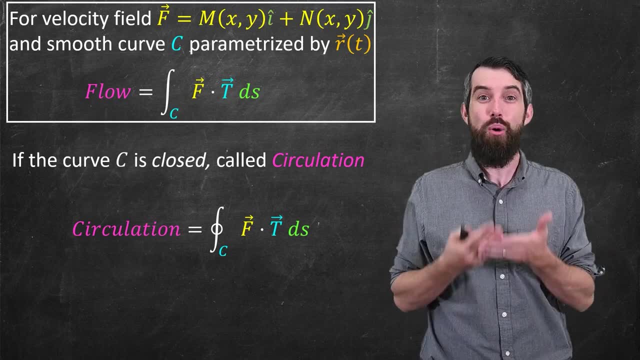 just indicates that it's a closed curve, And indeed, some of the concepts that we're going to see in this course are going to be dependent and only work when it's closed. So we're going to work when it's a closed curve, And so it's important to have this way to distinguish them. 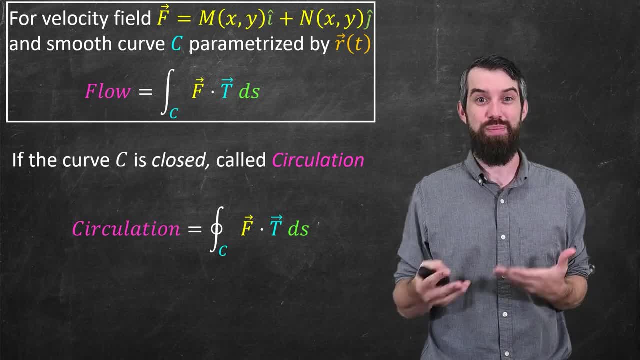 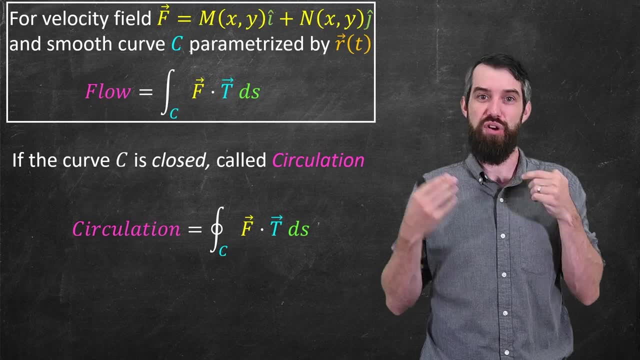 So when it's closed you put a little circle on the integral. Other than that, it's the same when we give it the new word, the circulation. So what is the circulation? The circulation is the total flow when you go around one loop of your closed curve. All right, so back to our two different 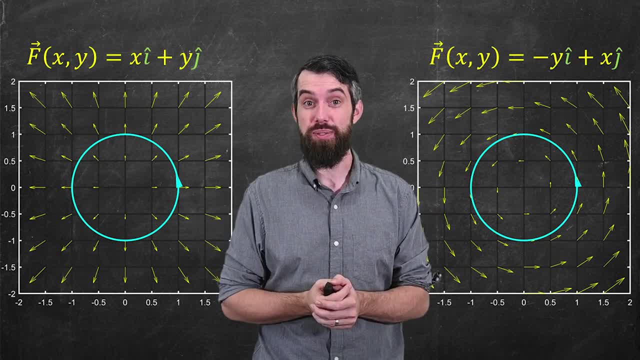 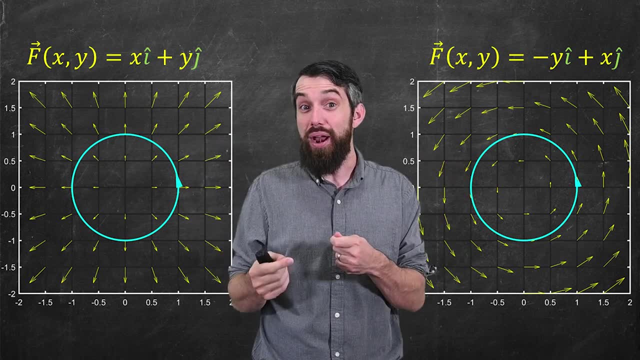 fields. What should we guess the circulation is in these two cases? Well, for this dispersion field, where everything's leaving from the origin, there is no spot at which the vector field is tangential to the curve Anywhere around this circle. for this field, it's the case that the 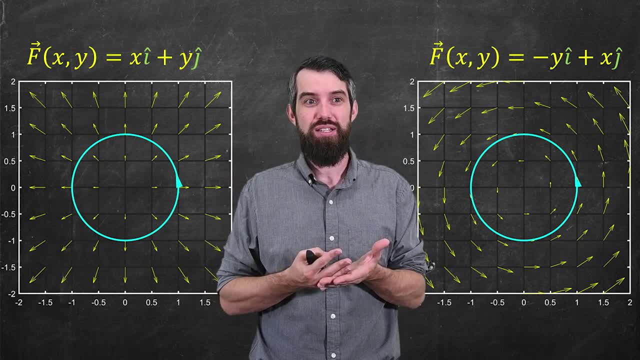 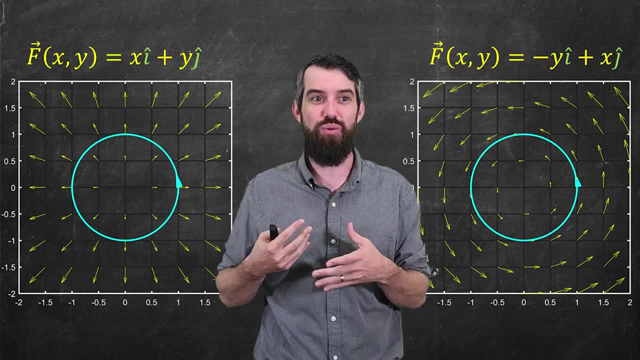 vector field is actually completely normal to the curve. So if you're thinking about what the flow does, flow is a measure of the degree to which you go along with the vector field. It's the degree to which, if you're in a canoe, you don't have to paddle but you're just flowing along the river. 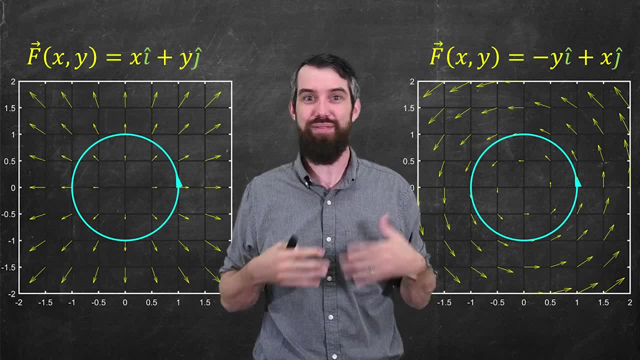 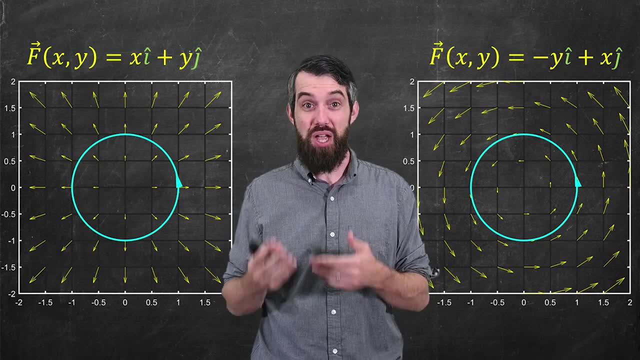 with the velocity flow of the river. Well, in this case, since everything's normal, that never happens, And so there is no flow or no circulation around the entire curve. In contrast with this case, at every point the velocity field is tangential to the curve. 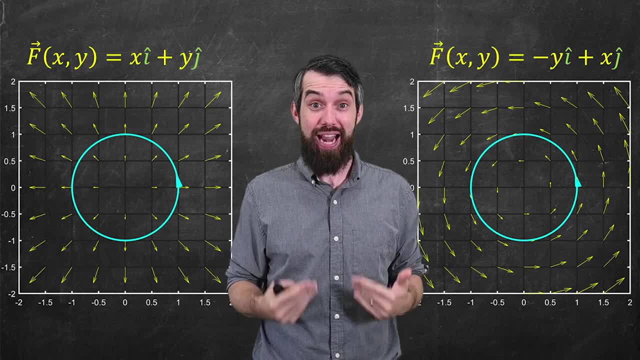 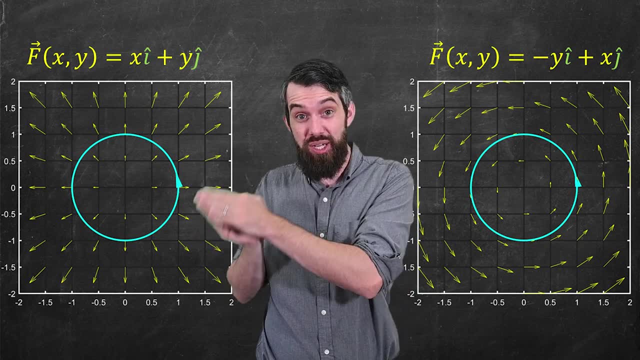 So we're going to have a lot of flow. the exact number we're going to have to figure out. So I'm actually going to ask you to pause and go and compute. what is the circulation in each of these two cases? The one I suggested was zero, but prove that to me. And then the other is going to 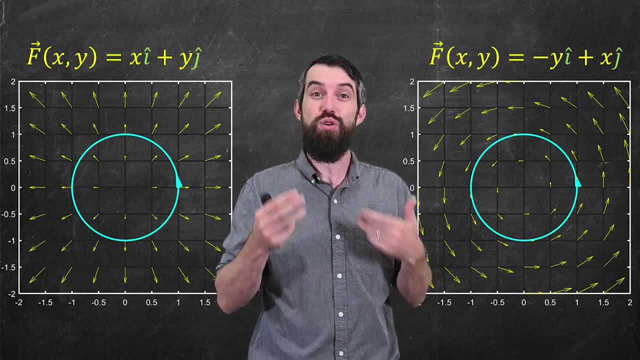 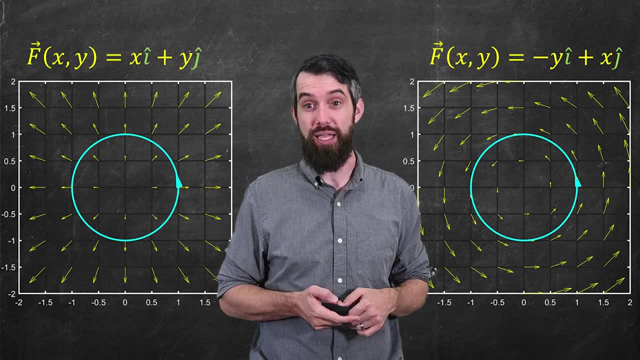 be some positive number. What number is that going to be? So I'll give you a moment to go and compute that. But if you just are here to watch the show, then well, let me walk through the first of them here. I'm going to begin with the XI hat plus YJ hat field, the one where everything's dispersing. 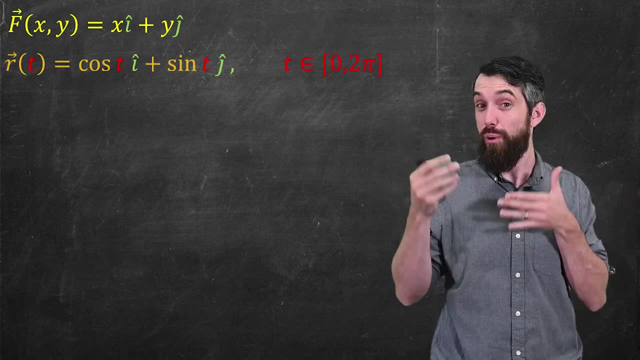 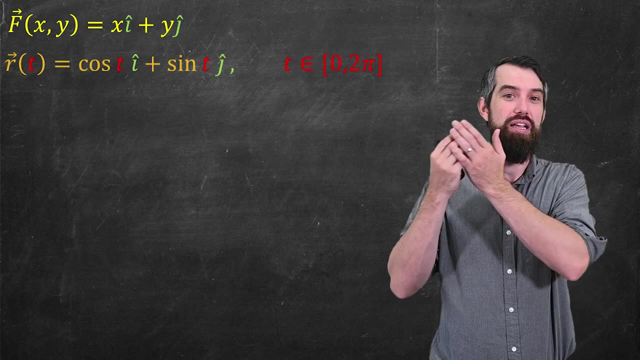 from the origin. I'm going to first, as I always need to do, parametrize my curve. This was the standard circle, So my standard parametrization for the circle is cos of T in the I hat, sine of T in the J hat, and T between zero and two pi. Don't forget, you always have to take the limits. 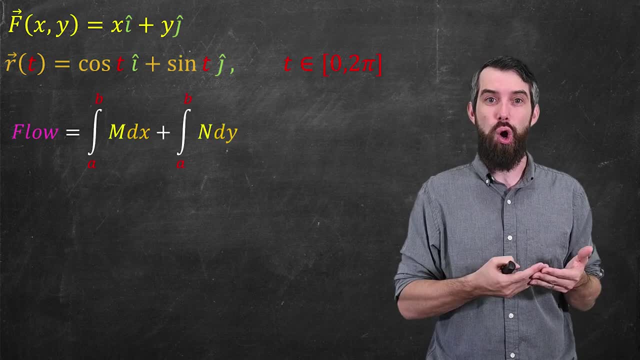 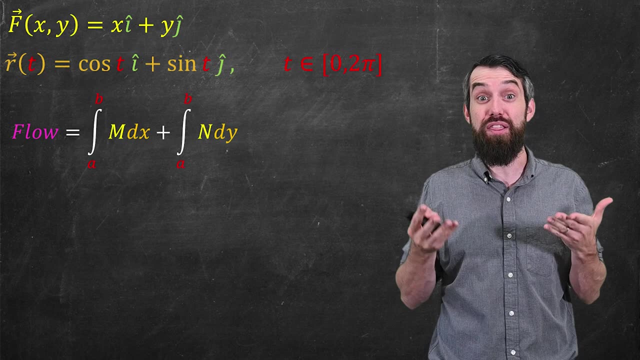 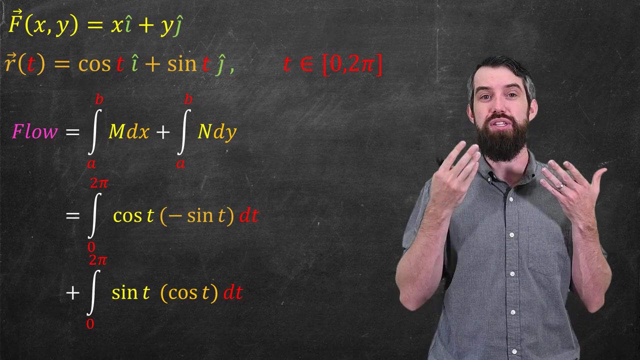 of your parametrization. The formula we had computed was that flow was the integral of MDX definition. but now I need to plug the values in. So M here is well. if I look at my field it was just X and X is cos T, So the M is cos T DX. I can replace with G prime DT If G is cos of T. 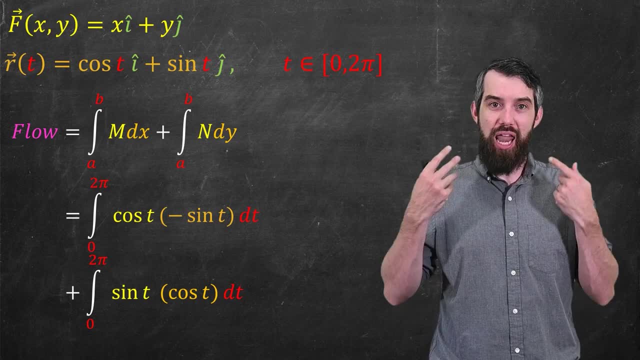 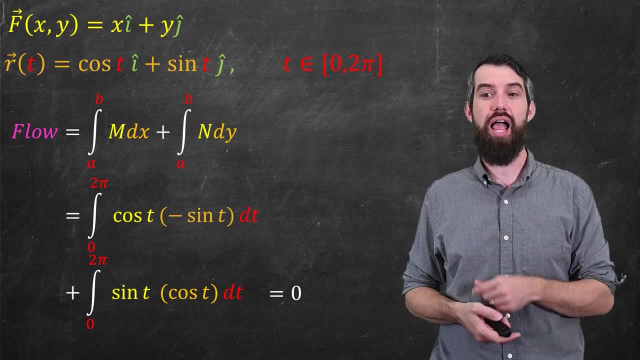 then the G prime is minus sine of T, DT, And then likewise for the integral of MDY. I'm going to have sine of T, cos of T And notice these are exactly the same, except for a difference of sine, and so they add up to zero. So, indeed, the field that we anticipated would have zero flow indeed. 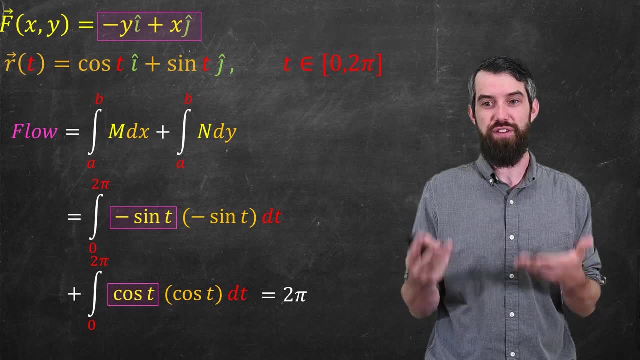 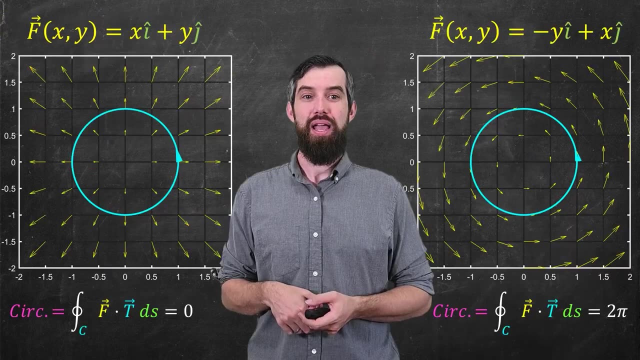 and then for the second one, you can walk through it yourself. I've changed the field here. It slightly changes the M and the N and gives the value of two pi. So where am I at? Well, I have my two different fields. For the left field, where the field was normal, to the curve at every spot. 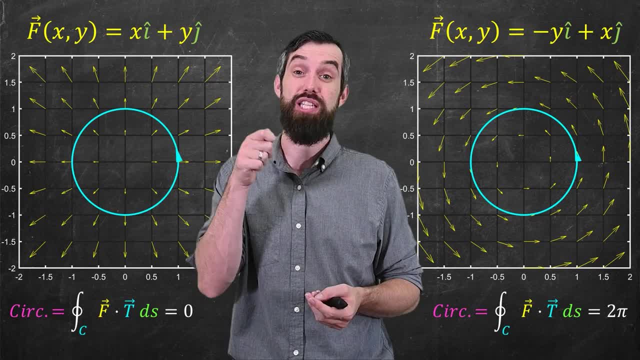 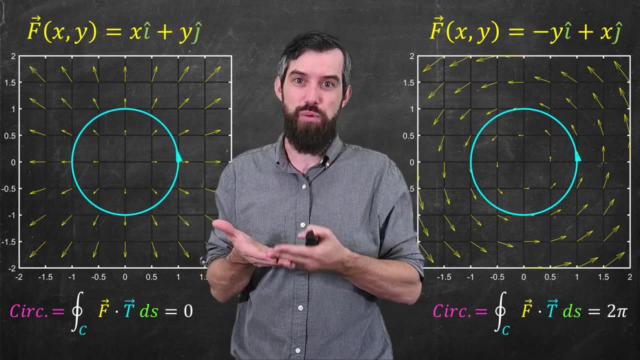 we managed to compute out that the flow- or since it's a closed curve, perhaps I should say circulation- was just zero. But for the spin field, where indeed we had these tangential field components to the curve at every spot, it actually added up to zero. So for the left field,